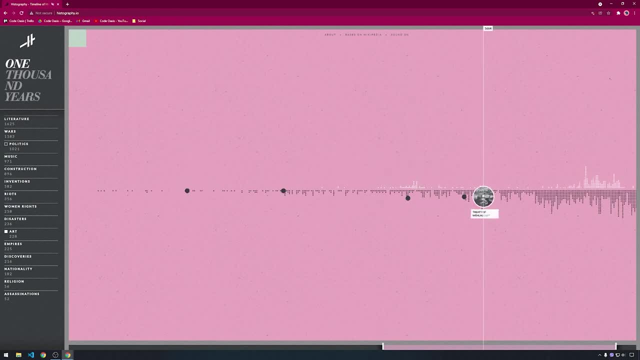 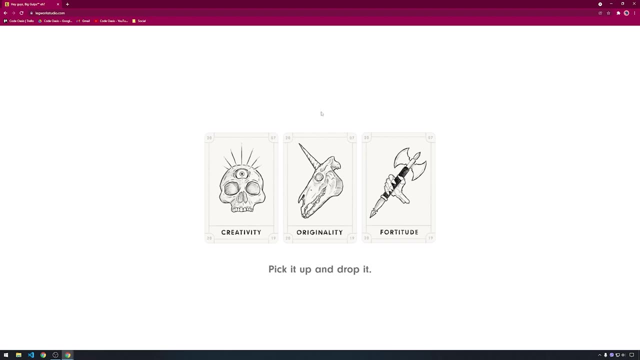 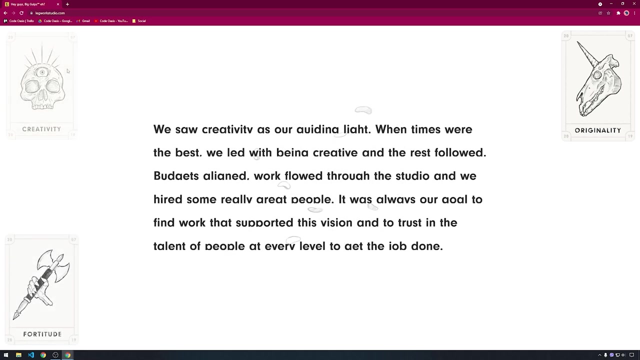 programming languages alongside Python and Java. Previously, it was mainly used for writing client-side applications, meaning that code written in JavaScript was executed in the web browser on your machine- client's machine. The introduction of Nodejs changed that, and now you can use JavaScript to write server-side code too, meaning that code written 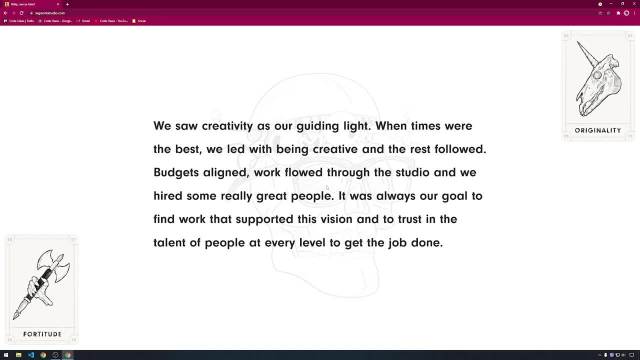 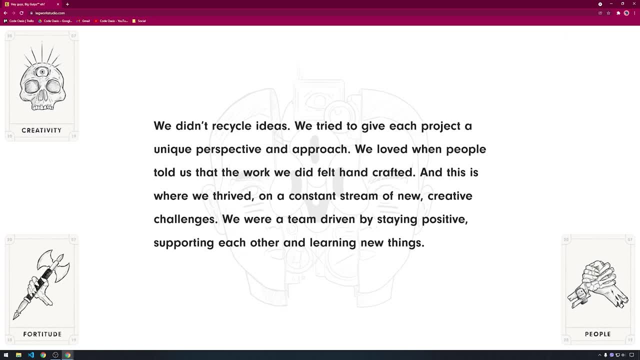 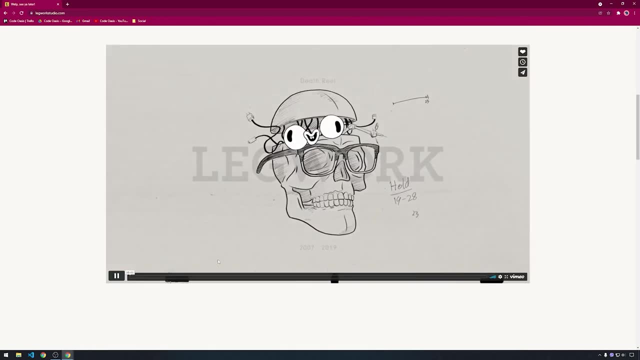 in JavaScript is executed on the server which is serving the application. Before Nodejs, JavaScript was also referenced as front-end technology, most often being used with HTML and CSS for creating websites, where HTML and CSS were used for website structure and styling and JavaScript was used. 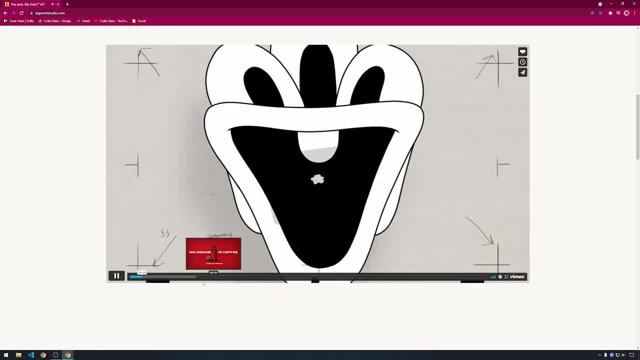 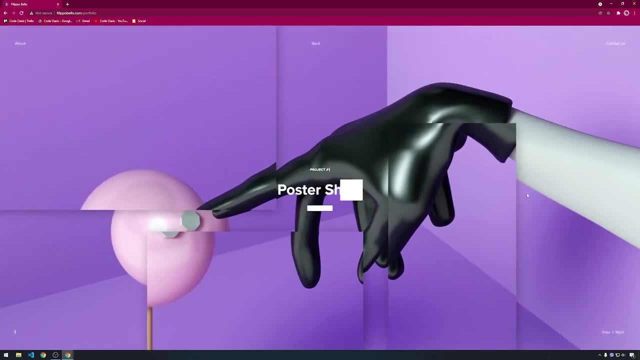 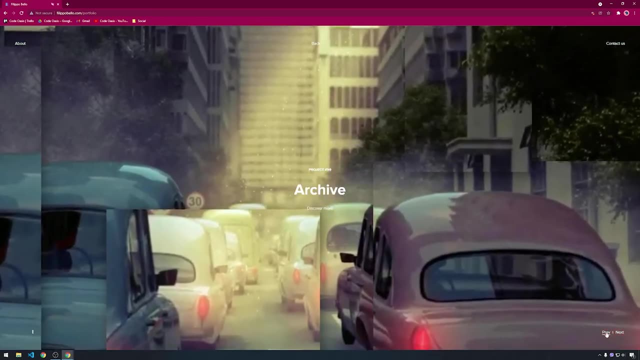 for all interactive, dynamic behavior which could happen on such website. To put it in concept, imagine that you have a button on the website. Code defining that button was written in HTML. CSS is used for button styling, making it appear in specific color and shape. 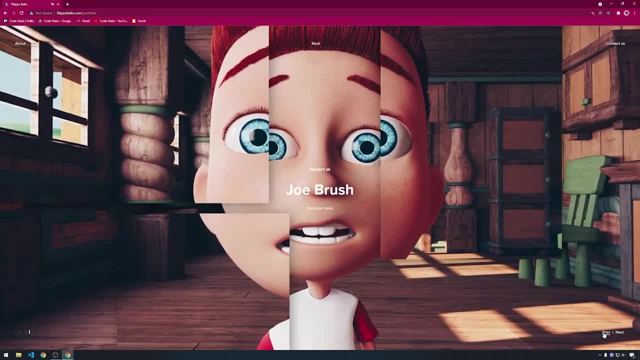 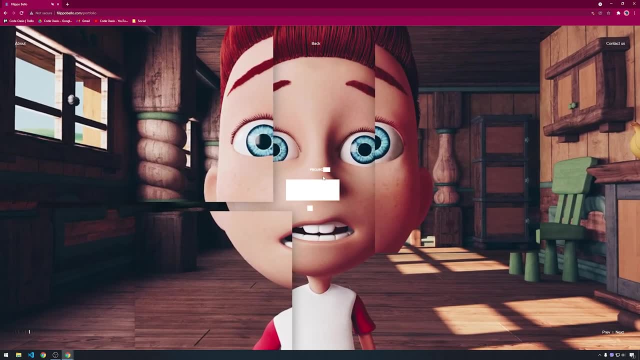 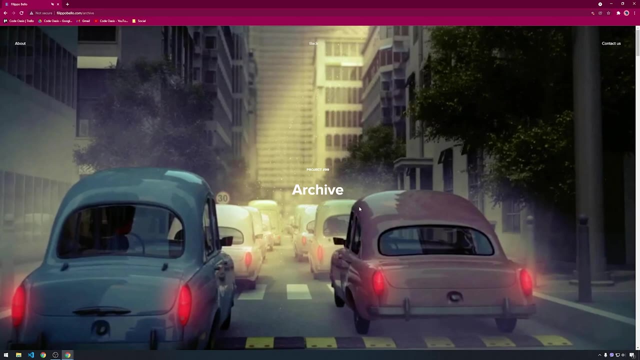 and JavaScript is used to define what will happen when you click on that button and how that button interacts with the rest of the website. Nowadays, aside from the already mentioned client-side and server-side applications, JavaScript plays a big role in mobile applications. There are also many popular frameworks and libraries written in JavaScript. In case that, 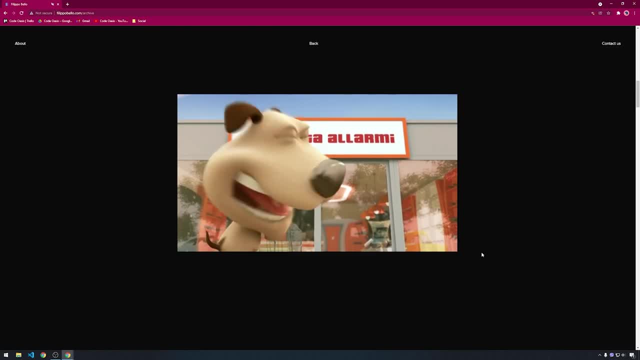 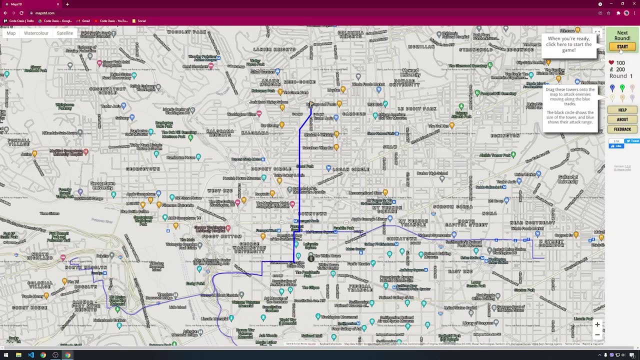 you're unfamiliar with the concept of framework or library, think of it as a set of tools and rules based on specific programming language, designed for speeding up the process of creating different types of code. If you want to learn more about JavaScript and JavaScript, you can. types of applications. So in case that you want to create some applications with JavaScript for web applications, popular choices would be Angular, React or even Vue For creating REST API. you might choose Nodejs and Express For creating mobile applications- good choices. 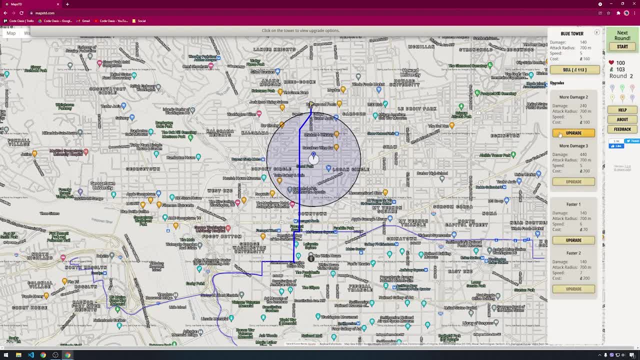 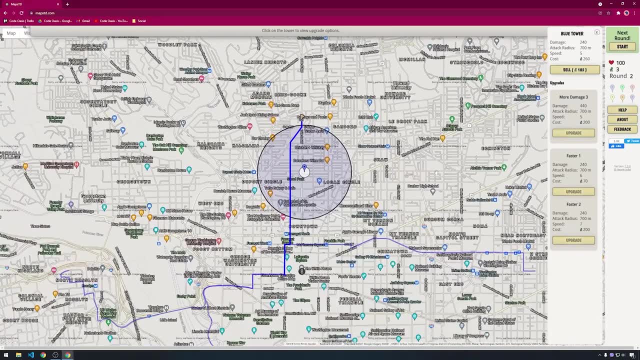 would be React, Native or Ionic. Let's jump to code and see some JavaScript in action. When it comes to JavaScript development, you have abundance of tools, But for now we only need a text editor and web browser. In theory, you could write JavaScript code in Notepad. 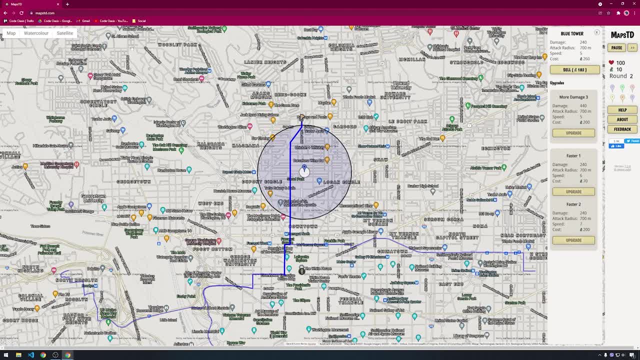 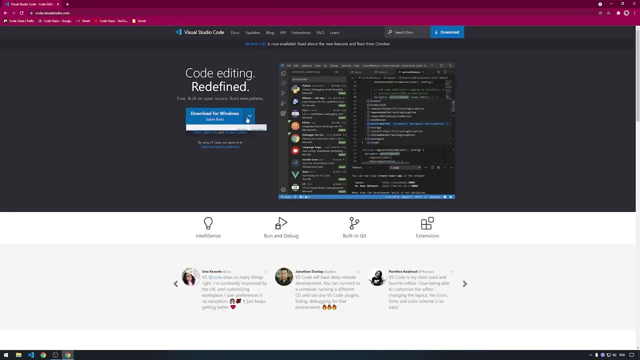 but since it's not very practical, my code editor of choice is VSCode. You can download it from here And I will also paste download link in video description. Installation is very basic, so I will not cover that part. If you need assistance there, google it. 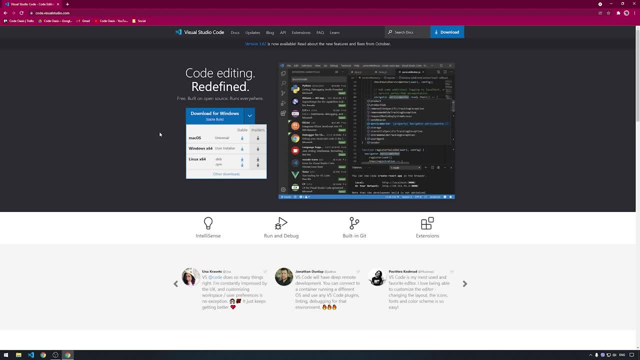 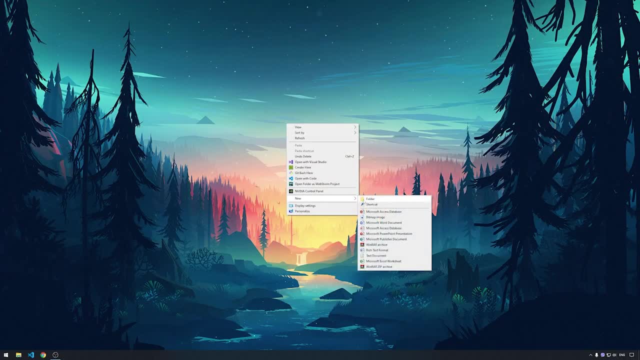 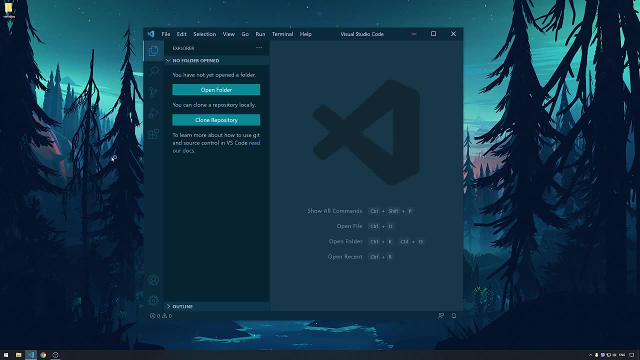 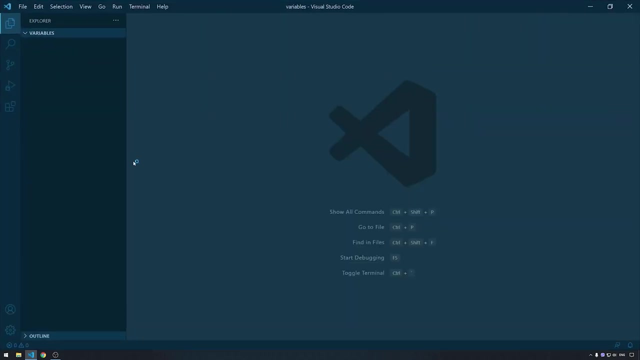 As I said, you will also need a web browser. I'm using Chrome. Now let's create a new folder. Call it whatever you like. I will call it Variables, since that is the topic of this video. After installing VSCode, open it and drag that folder inside. 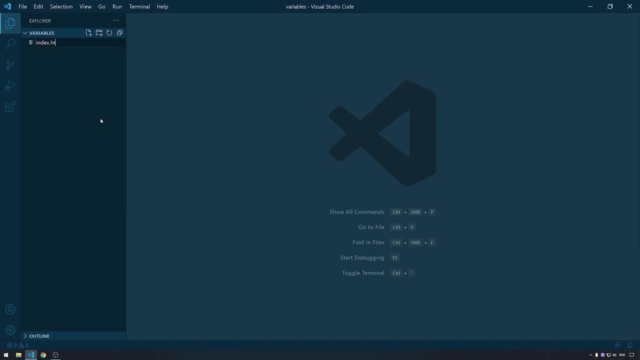 In VSCode, create new file and name it indexhtml. This will be an HTML file. It will be very HTML file, but we will use it only for hosting our JavaScript code. We need a few lines of HTML boilerplate code in order to be able to write JavaScript code. 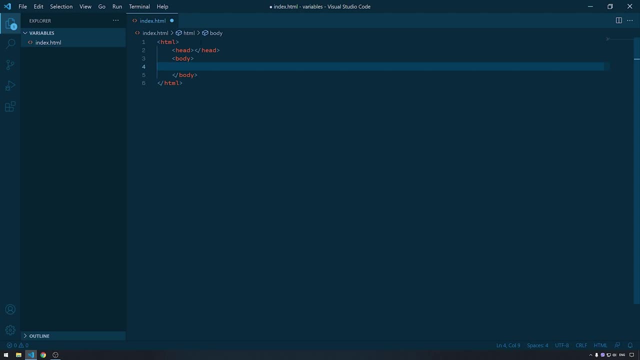 These are called tags and they represent starting and ending of any code block in HTML. Now we can write JavaScript code by adding script tag, and just to test it all out, I will write consolelog statement, Hit save. and now to see our code in action, we need to open this indexhtml file in our 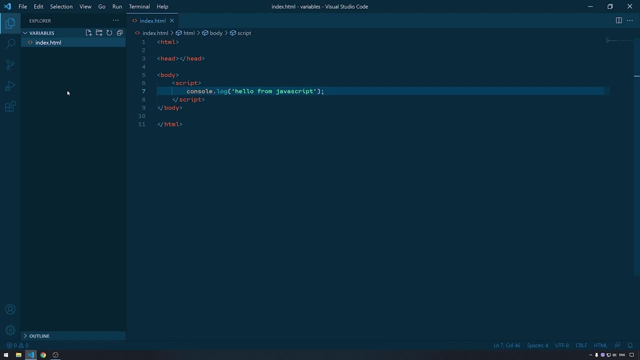 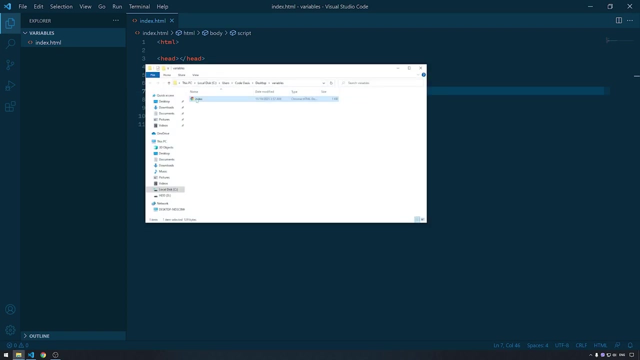 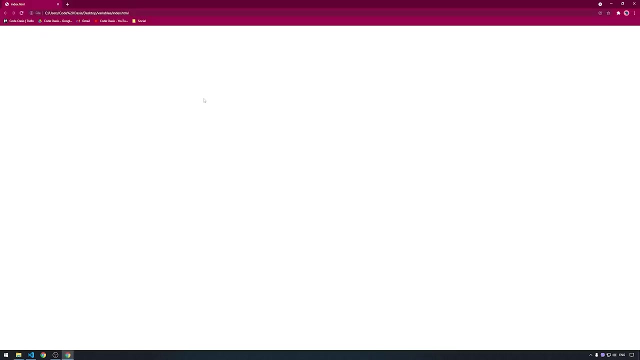 web browser. Fastest way to do so would be to right click here in explorer area of VS code and select reveal in file explorer. And here you can see our indexhtml file. Double click on it and it will open in your default web browser. 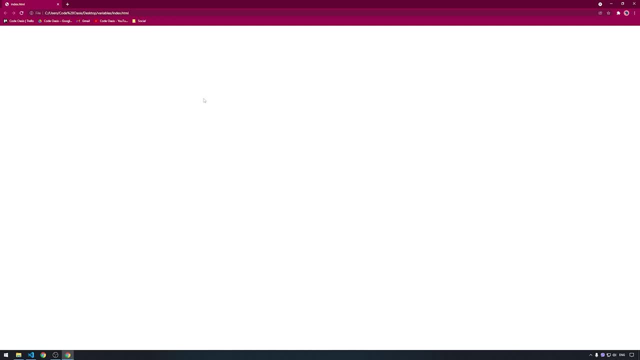 Now it might seem as there is nothing here to see, but that's because we didn't wrote any visible HTML code. What we wrote is JavaScript consolelog statement and it can be seen in developer tools. To open developer tools, press F12 or function key plus F12, depending on your keyboard. 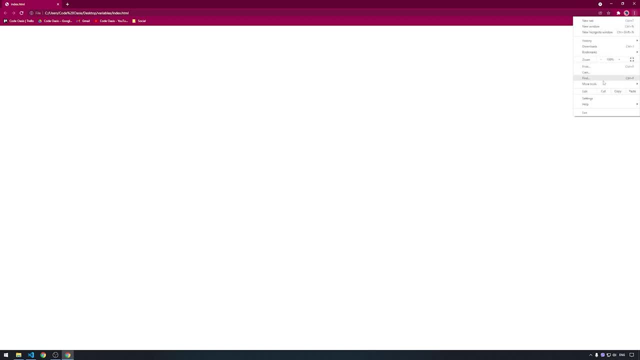 You could also navigate using your mouse to browser options And look for developer tools. When you open developer tools, select console tab if it's not already selected. If you successfully navigate to developer tools and you can see a message: hello from JavaScript. be proud, it is your first JavaScript application in action. 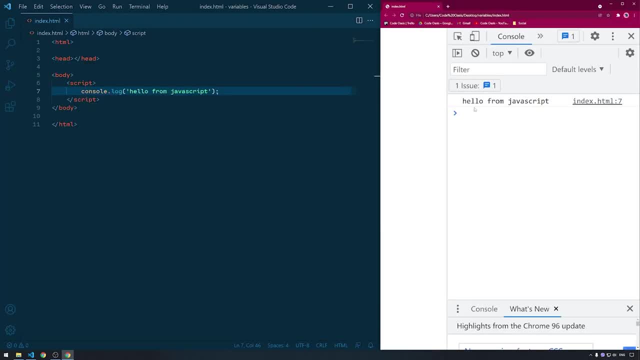 It doesn't do much, but still congratulations. now we can do some serious work. That single line of JavaScript code is called a statement. You can think of statements as a list of instructions Executed by the computer. Every JavaScript application consists of list of programming statements. 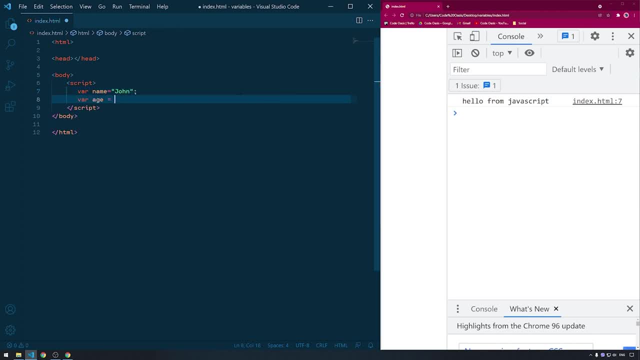 These are also statements, but they are variables too. So what is variable actually? Imagine that we have user called John who happens to be 29 years old. Now imagine that it is some information which will be used by our application. So for our application to remember that information, we have to store it somewhere. 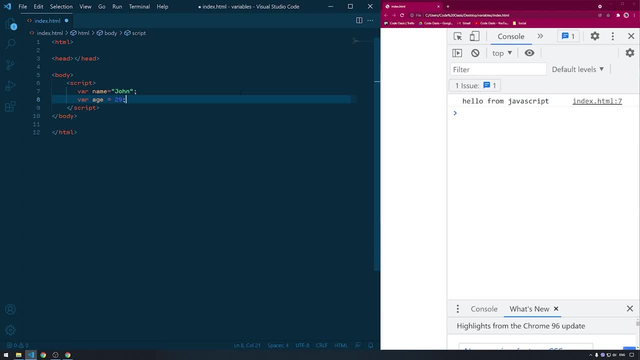 And for that we use computer memory. A real world example would be a fridge with many cans where each can holds some sort of food. It wouldn't be very practical if you had to open every can just to know what kind of food is inside, right? 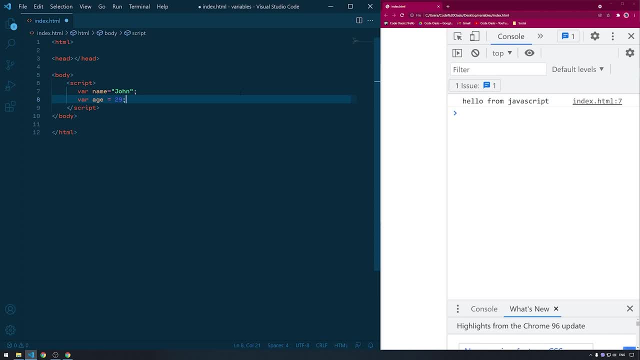 That's why each can have some sort of label. Well, computer memory is fridge, can is memory address, and variable is just a label letting us know what piece of information we want to store. So this is a data set of information is stored on that address. 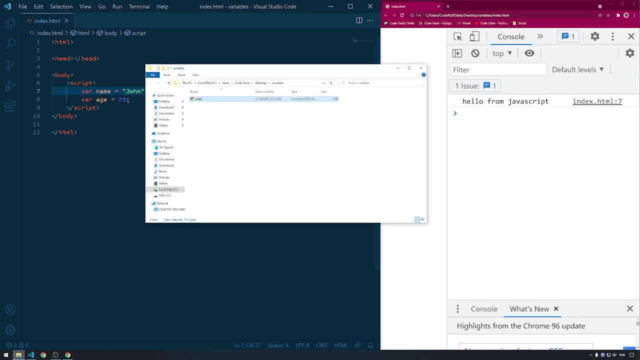 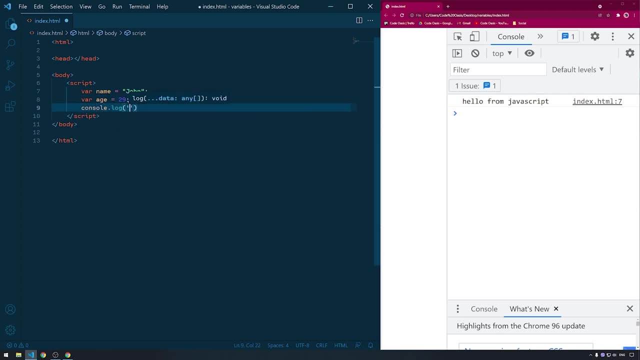 Now, if we want to use this set of information in some meaningful way, we could write something like this: Go back to Developer Tool tools and refresh the page. You should see the message that says my name is John and I'm 29. 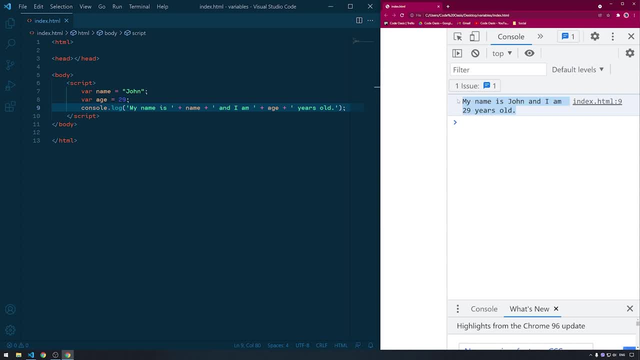 years old. This statement is simple but nice example that can help you to see how we can construct information that we are showing to anyone who is using our application or, as you will often hear, to so-called end users. Let's analyze this statement a bit more: Console log. 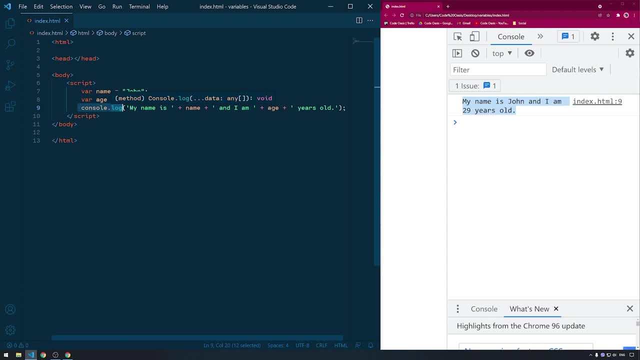 is one of many JavaScript tools. It is used to quickly show the current state of data in developer tools, and I say current because data can and most likely will change during our application execution. This part is called string. String can be any set of characters inside double. 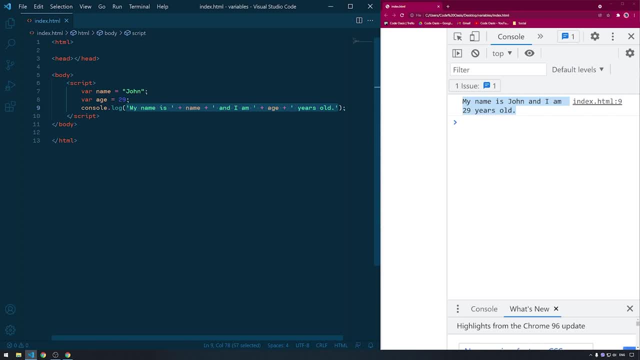 or single quotes. We can also see that we constructed this string by using both static and dynamic parts. Static parts are those inside quote quotation marks, And dynamic parts are variables because their value can vary, hence the name. So anything that can change the value during application execution should be stored into. 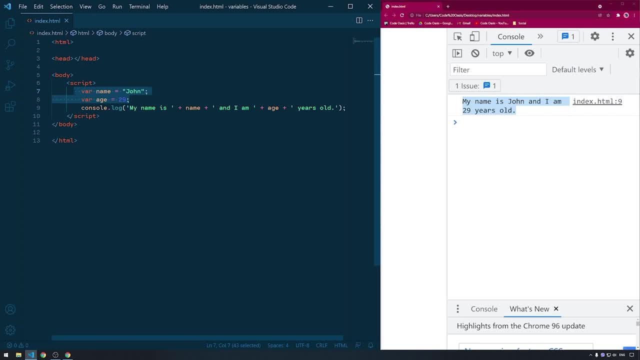 variables. This means that everything stored inside quotation marks JavaScript reads, as is. But when it comes to variables name and age- JavaScript knows that those are variables. So instead of writing out just plain word name, it looks into computer memory and finds address which variable name points to, and then reads data. 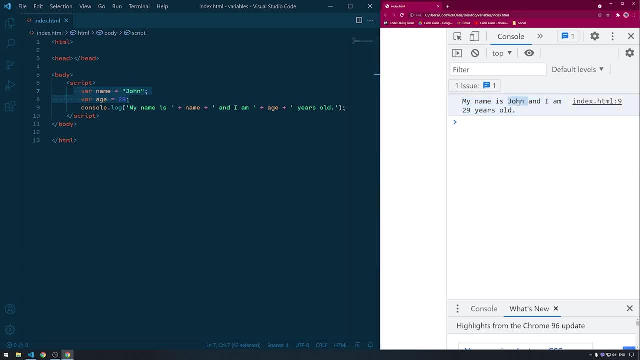 stored on that address. That's why we see John instead of name. The same applies to variable age. We could even store this entire message into variable, like this, And then we could say Go back to browser and hit refresh. As you can see, the result is still the same. That is because message is now a variable and JavaScript will look in memory for an appropriate address that is tied to that variable and read data located on that address, even though data consists of other variables pointing to other memory addresses with other pieces of data. 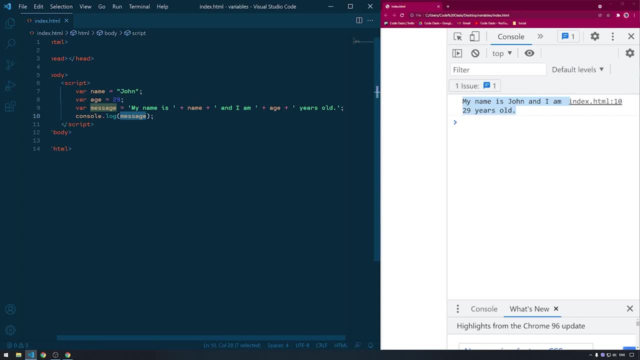 Before we go any further, let's quickly improve our efficiency. Instead of manually refreshing page in web browser every time when we want to see changes that we created in code, we could use an extension called live server. Go to Visual Studio extensions. Type live server. 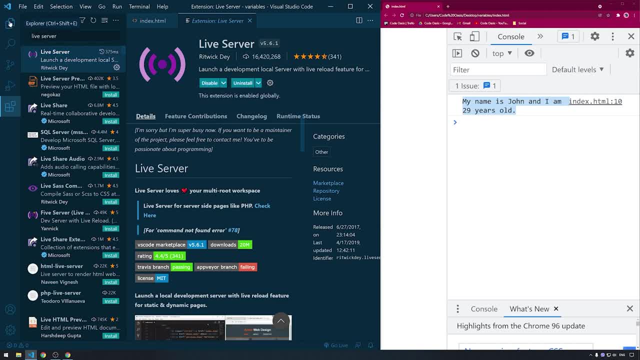 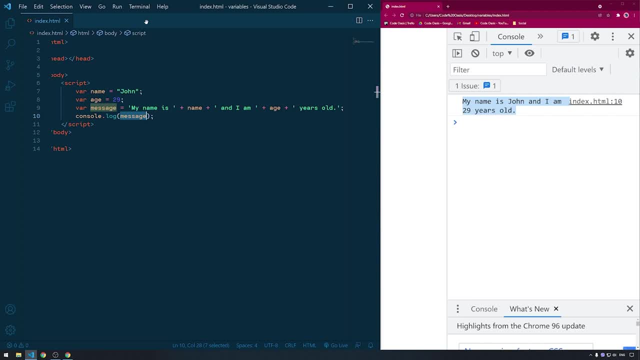 And install it. What it does is that every time when we save changes in our code, browser page will be automatically refreshed. Neat right Once it is installed, click go live and it will open our application in your default browser, Same as we did manually at the beginning. 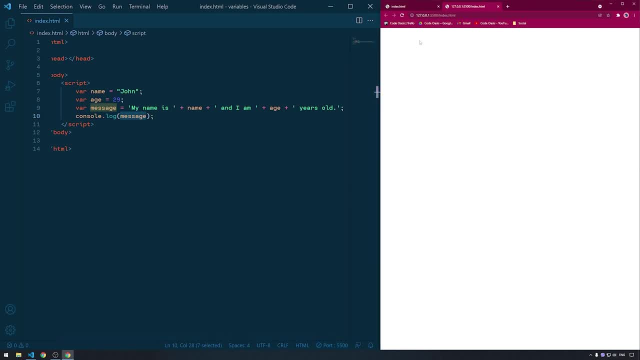 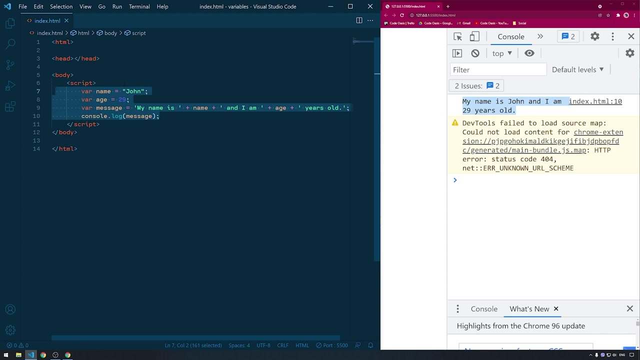 If you don't see this go live option, simply reopen your VS Code instance and it should be visible. We can close now our old tab. Now I will comment out this previous part of code. Comments are useful for keeping short reminders and explanations of certain pieces of code. 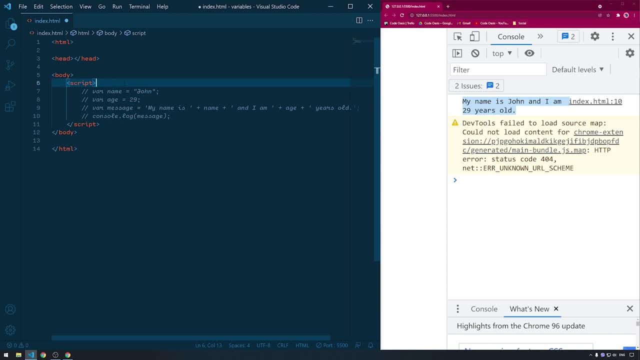 Think of it as your personal notes, or notes that you left for other developers that are working with you on the same project, So I could also write here something like old examples and new examples. Everything that is under comment will be skipped by JavaScript engine, meaning that it won't be executed as the rest of the code. 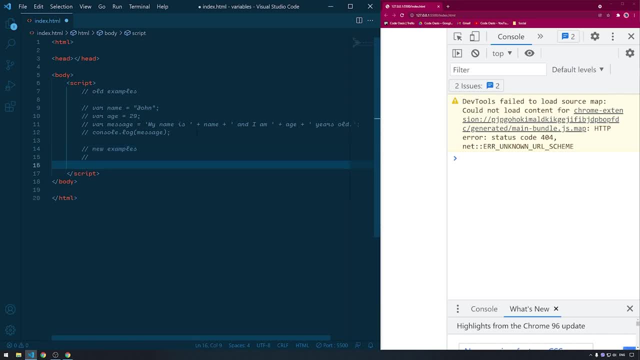 You can write single line comments with the same code, Double line comments with double slash, or multi-line comments with slash, star, star, slash. So multi-line comments would be something like this. I know that I have mentioned JavaScript engine. Think of it as part of your web browser dedicated to executing JavaScript code. 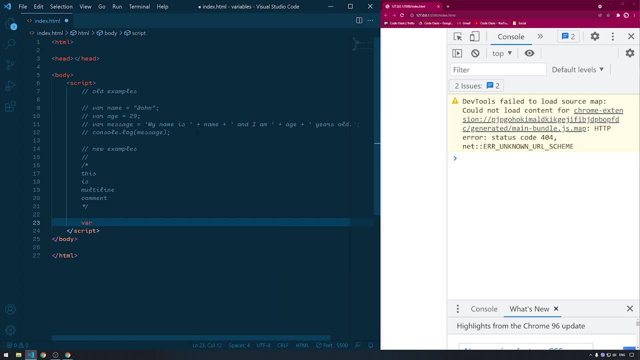 Previous variables we declared with keyword var. Var simply indicates variable Aside from keyword var. in newer versions of JavaScript we can declare variables with keywords let and const. There are many differences between those three, but for now remember only this: Variables declared with var or let does not have to be initialized at the moment of declaration. 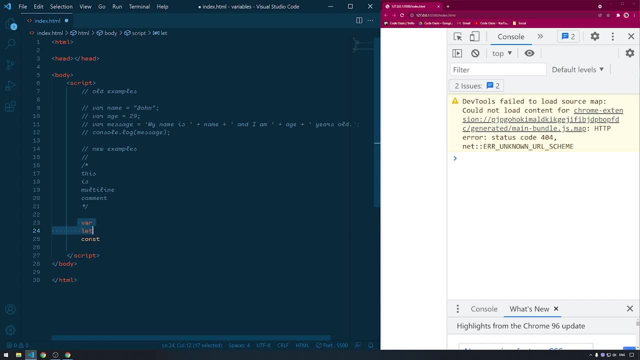 And they can also change value later during code execution, Whereas variables declared with const can have only one value And it has to be assigned at the declaration time. Just to clarify: declaration is creating variable like this, And initialization is assigning value to that variable, like this. 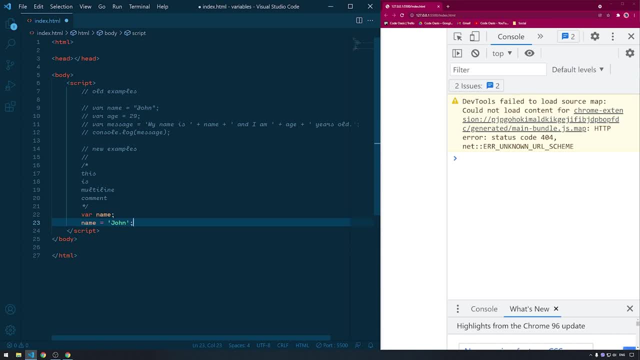 Now, with var and let variables we can do it both at the same time, like this, Or we can declare variable and then later assign value. With const variables we have to do it at the same time. We have to do initialization and declaration at the same time or the application will break and we will get error in console saying exactly that. 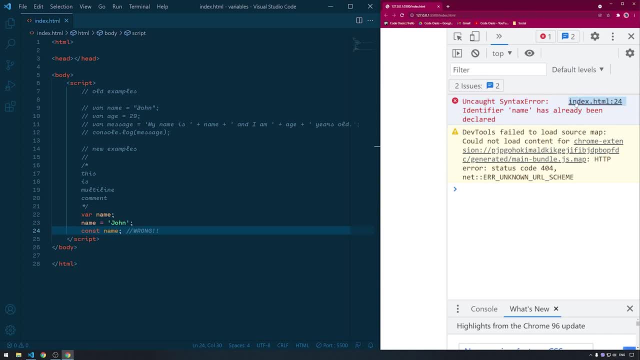 Aside from that, the error log shows file and line where that exact error occurred And if we check our code we can see that is part of code when we declared but not initialized our const variable. Now if we change this line to this, We can see that error in console is gone. 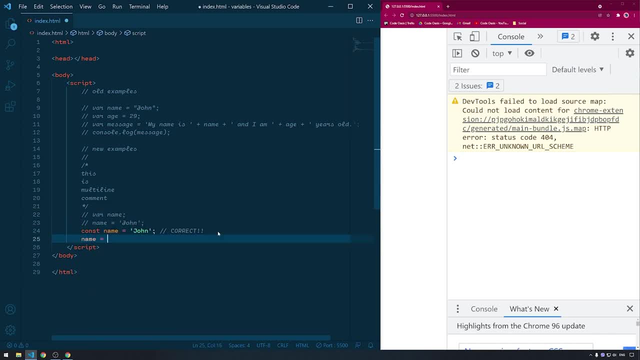 Once const variable is initialized, if we try to change its value, we will also get an error saying that we cannot change the value of constant variable. If we comment last line out, error is gone. Now a few words on types of data that you can store into variable or, to be exact, into memory location which that variable points to. 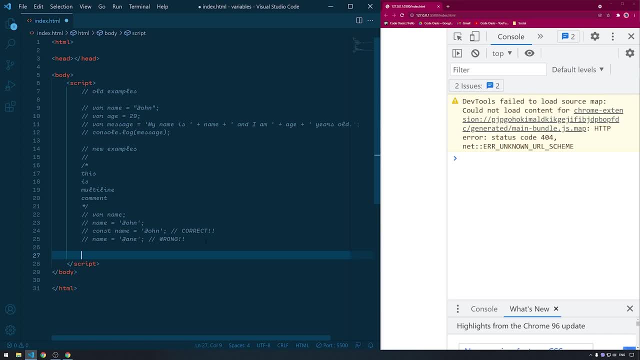 All data types in JavaScript are divided into primitive and reference data types. Reference data types will be covered later in this course. Primitive data types, aside from string, are number boolean- undefined, and null. String can be represented as one or multiple characters inside quotation marks. 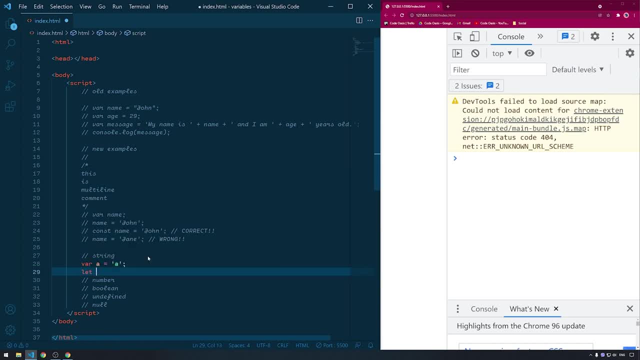 This is string. This is also string. Number can be represented with integer or decimal values. Notice that numbers are not inside quotation marks. If they were, They would no longer be numbers, but instead they would also be considered as strings. So this is actually a string, not a number. 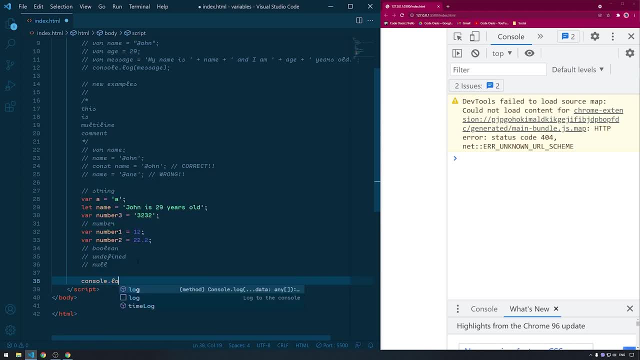 To check the type of some variable, we can use another built-in JavaScript tool called typof. Variables can also hold boolean types of data, meaning that they can only have values of true or false. We can see that type is boolean. We also have null and undefined. 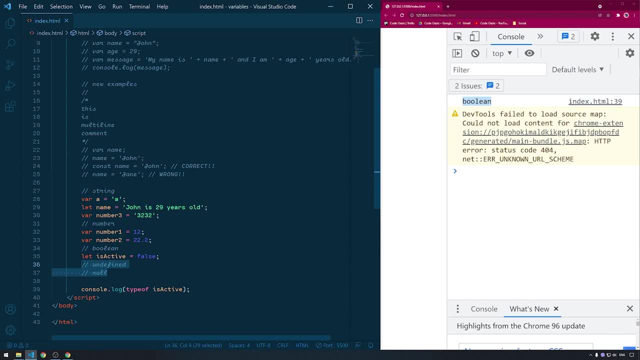 Undefined simply means that value of variable is not yet defined, It does not exist, whereas null is by itself already a value, but that value is empty. Is that confusing? Think of it like this: Here you can see that value is explicitly set to null, but if I remove initialization, 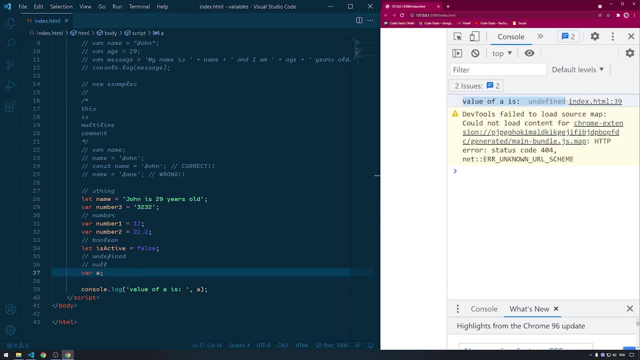 you can see that value is undefined, So you want to use null when you want to explicitly define something as empty, whereas undefined usually means value was never assigned or there is some sort of error. Let's make this a bit more interactive. You can declare variables together too, like this: 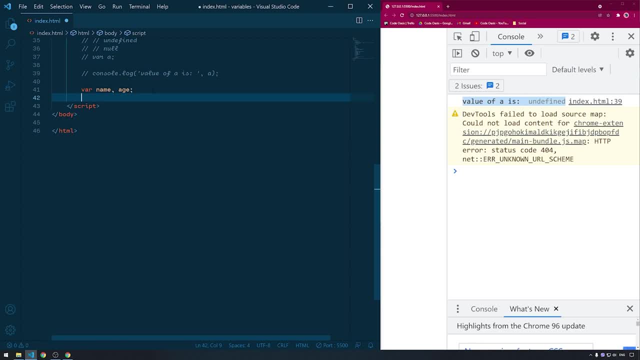 Now we use another JavaScript tool called prompt. It is used to capture user input during the runtime of application. Runtime simply means while your code is executing. So we are politely asking our end users to enter their name in our application, We are doing the same for variable age and finally, we can output that data that user entered in form of pop-up window. 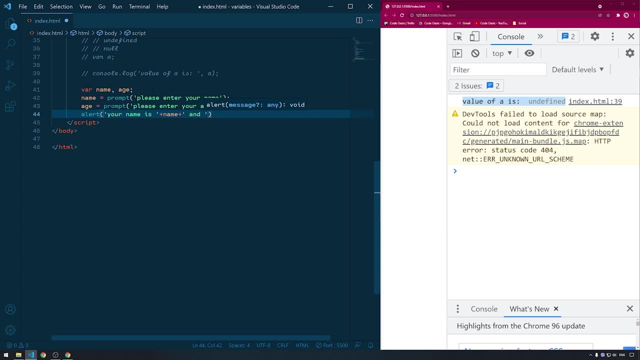 For that we are using JavaScript tool called alert. Think of it as opposite of prompt, It outputs information instead of receiving it. Hit save and witness the magic. Now you can see that the code is working in browser. Another quick example would be writing code for performing some mathematical operations. 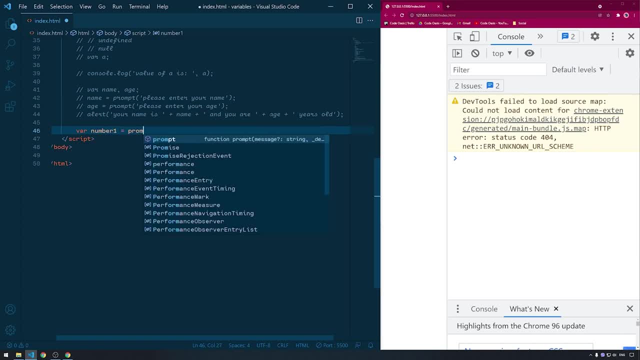 You could write something like this: He would show the input. Now I will generate the input. You can see it is now working. Then you have to create the code for their last ¿¿$¿. Also, you can create there as well. 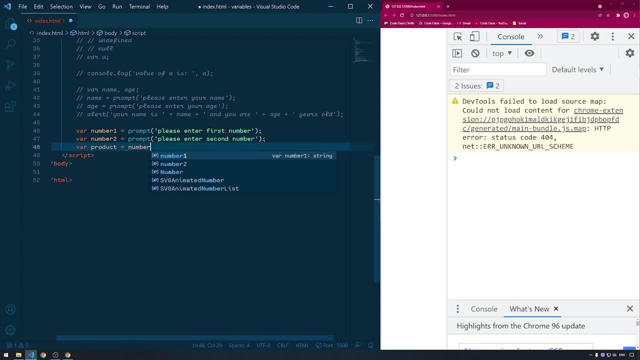 It will send me the code and I will add my own code. Once we have created that code and we are done with the application, You can now call it on the cloud. You can see the code has been created If I go into my browser. 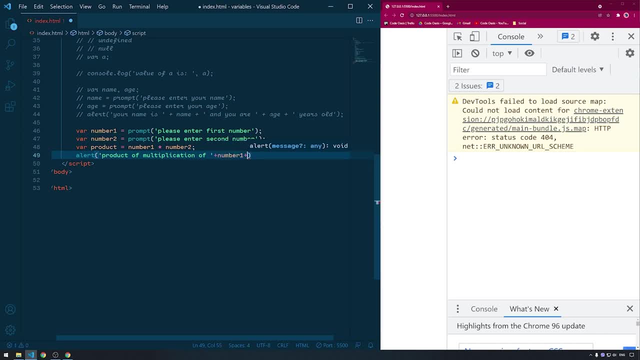 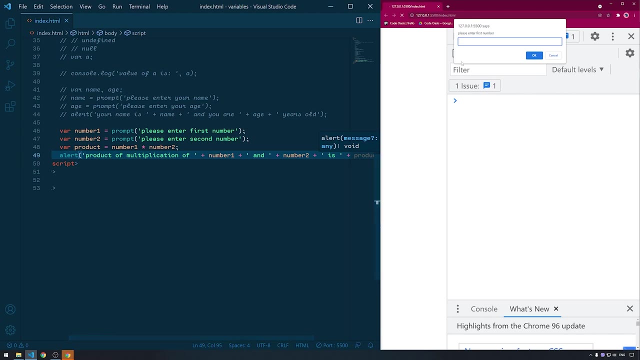 If I go to my social network or website Then you can see the code for my application. So you must like and subscribe to my blog. So it is Again magic in browser. There you can see how easily we can make an interactive application that receives some 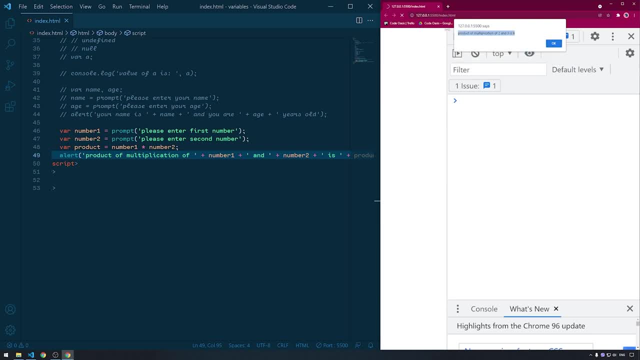 sort of input data and based on that it produces some sort of output. That is, in a nutshell, how pretty much every application works. When it comes to naming variables, we must obey certain rules. Here I will just copy that set of rules from V3 schools. 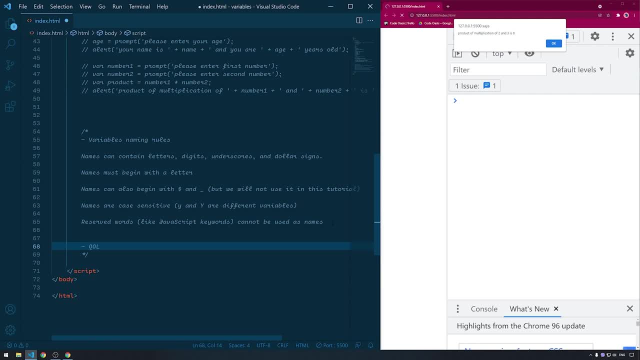 To this list I would also add few things which are not strict rules, but more like quality of life advices. When naming a variable, try to use descriptive, meaningful names. It will save you a lot of trouble when it comes to writing big applications with hundreds. 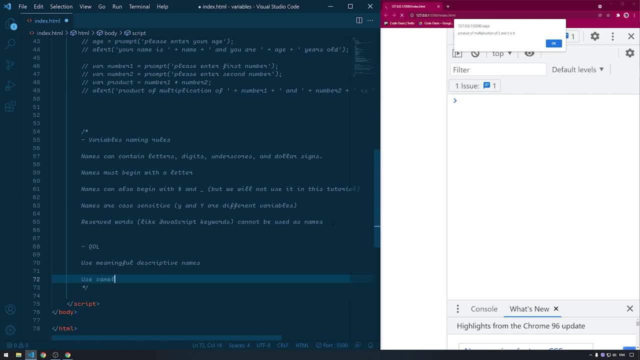 if not thousands of variables. Use naming conventions such as camel case, For example. if you want to create a variable for date of birth, since you can't use spaces, camel case notation dictates to write it as date of birth. As you can see, the first letter is lowercase and every new word is represented with uppercase. 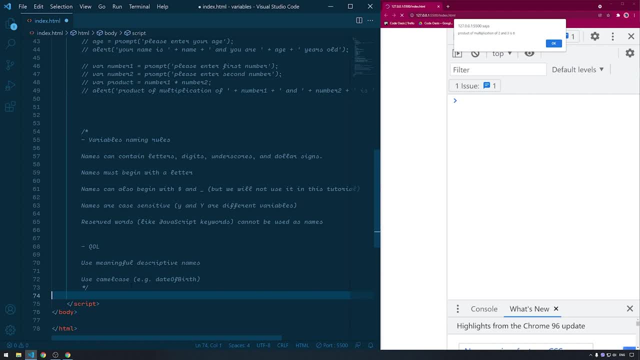 Since JavaScript is dynamically typed language, it means that type of variable is determined during runtime. Remember what we said: During runtime, This simply means while JavaScript engine is executing your code. This provides many possibilities, but it also can create some confusing situations. For example, in JavaScript, you can say something like this: 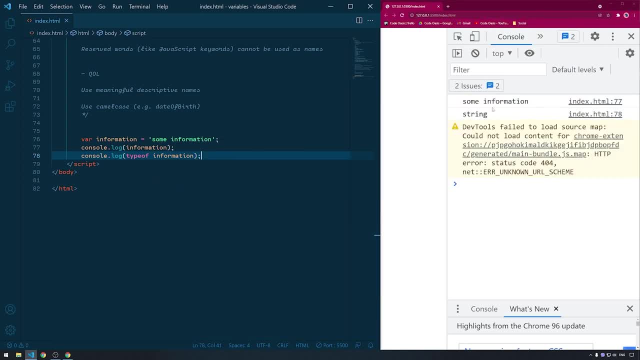 Now, when we check, we can see that value is some information and type of this variable is a string. Now we can say: information equals 45. If we check again, value is 45 and variable type is number. now Here you can see what I meant when I said that type of variable is determined during. 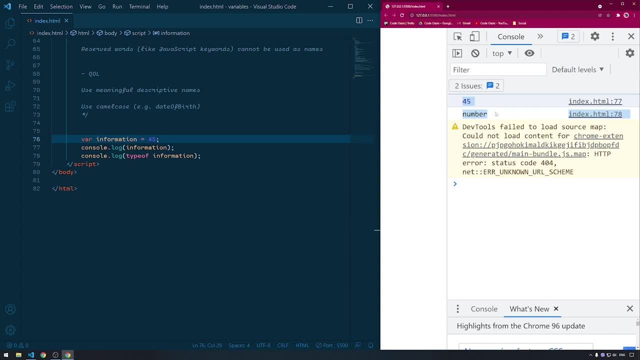 runtime, Depending on value that we assigned Variable changed from string to number. If we change it back to some information and say something like this, JavaScript will concatenate these two strings into one. If we change variable to 45, JavaScript will still combine those into string. 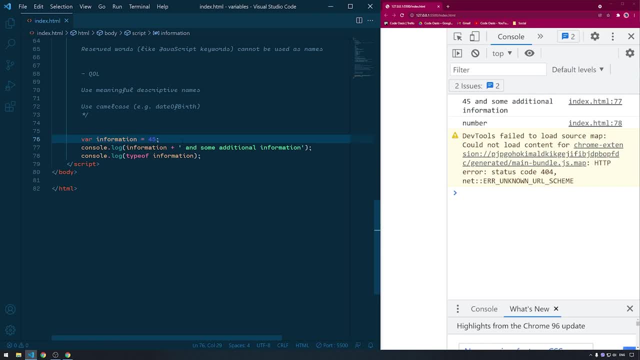 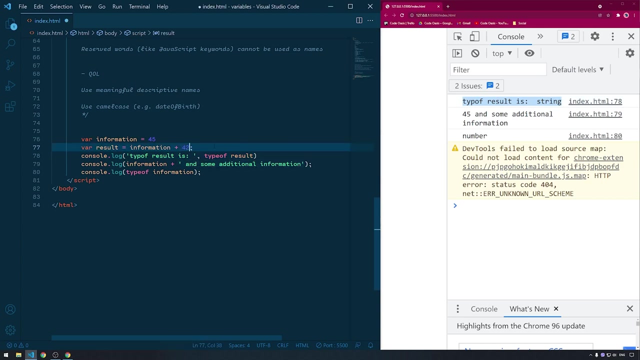 We can check that by storing result of this concatenation into variable like this: Now you can see in console that it is really of type string. But if we change it to this, could you guess what will happen? now JavaScript figured out that both variable and static part. 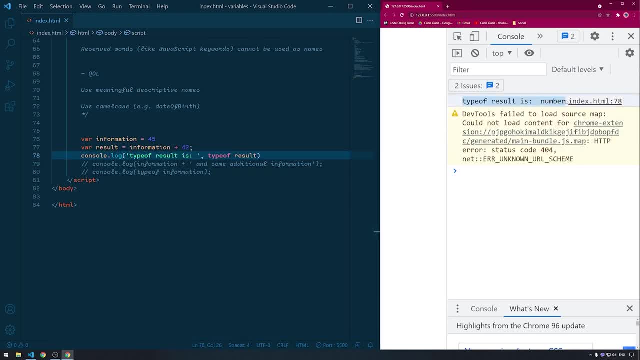 are of type number and result is no longer string but number. But that's not all. Result is not number 4542,, as you might expect, Since both parts are numbers. if we put plus between, it won't concatenate them, but it will summarize. 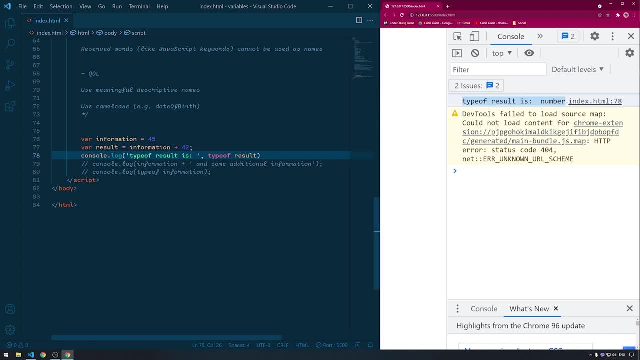 That's just how JavaScript works. But if we change it to this now, the result will be 4542, and type of result will be string. That's because, once again, JavaScript is smart enough to know that variable information is now type of string. 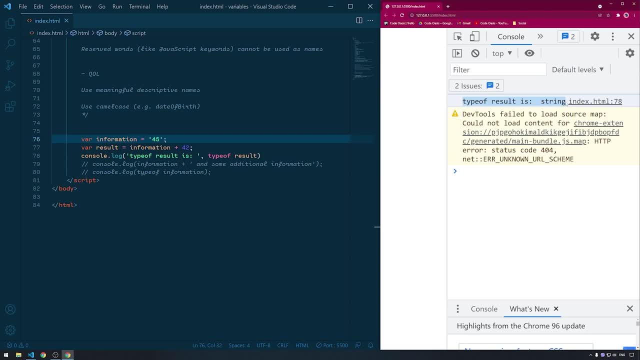 And it won't try to summarize string and number, because it doesn't make sense. You can't perform mathematical operations on words or letters, So it will instead transform everything to string and concatenate it If you for some reason want to change type of this information. 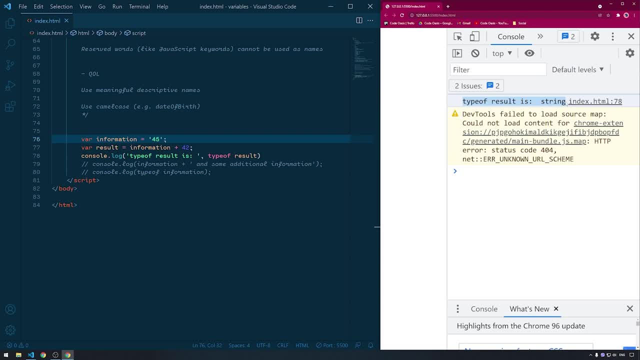 variable. at the moment when this line is executing, you can cast it to number. Casting simply means changing one type into another. You do that by adding plus sign in front of it like this. Now again, type and output changed. Difference is that type of variable information. 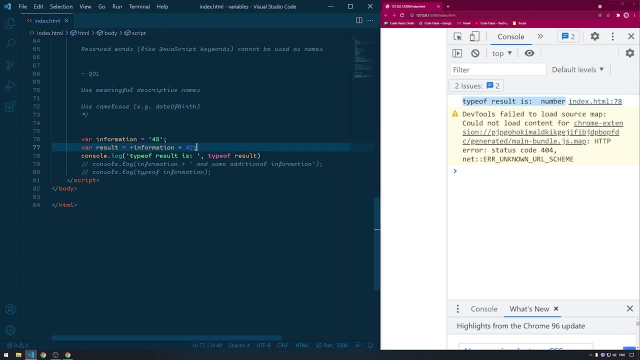 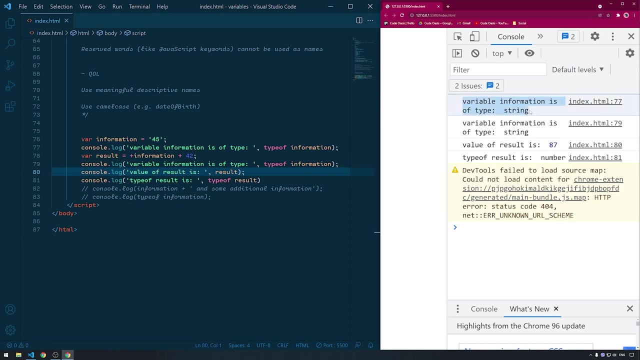 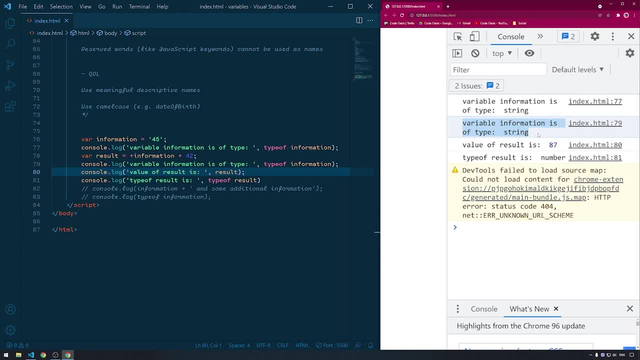 If we add a couple more of console logs, we can see that. OK, I will stop here for now. As with every topic, there is a lot more to say about variables too. But for starters this is enough, because this is only first part of many to come.